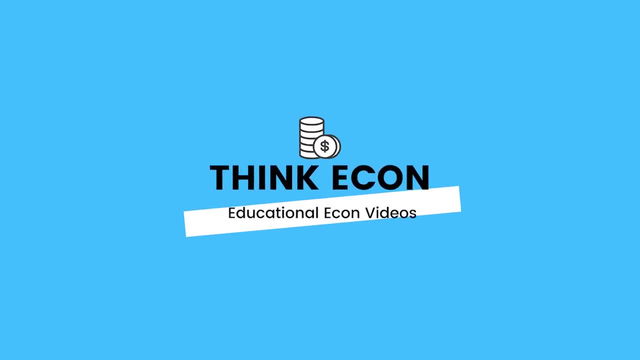 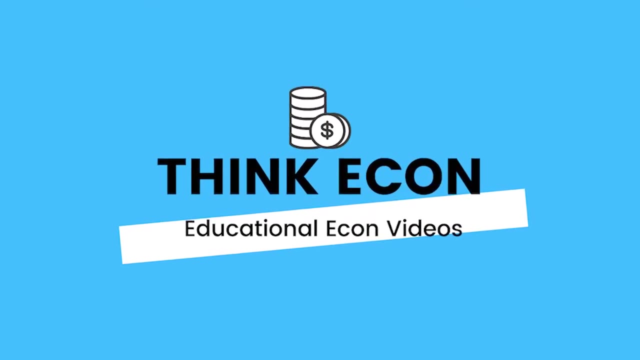 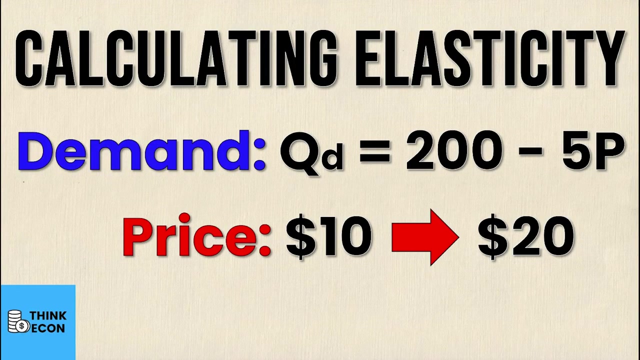 Hey everyone, and welcome back to the channel. In this video, we'll be reviewing how to calculate elasticity of demand, given nothing but the demand equation and a change in price. With that said, let's get into it. So, as promised, in this video we'll be calculating the elasticity of demand. 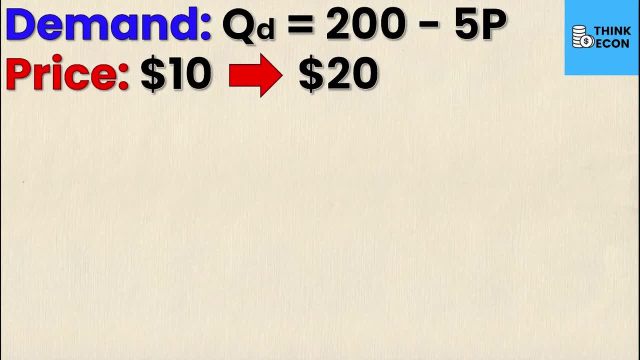 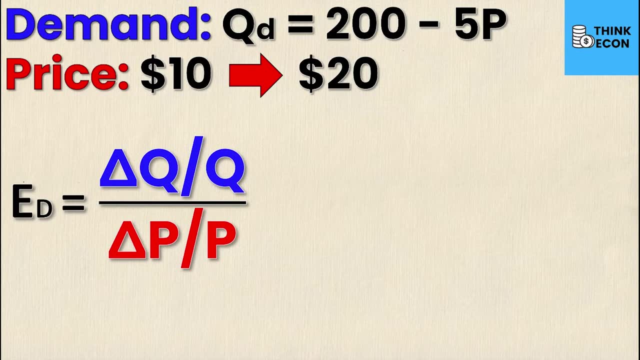 and to do that we need to remember the formula for elasticity of demand, and that's simply the change in Q or the change in quantity divided by quantity, over the change in price divided by price. And for this formula to work you need two different prices and two different quantities. So 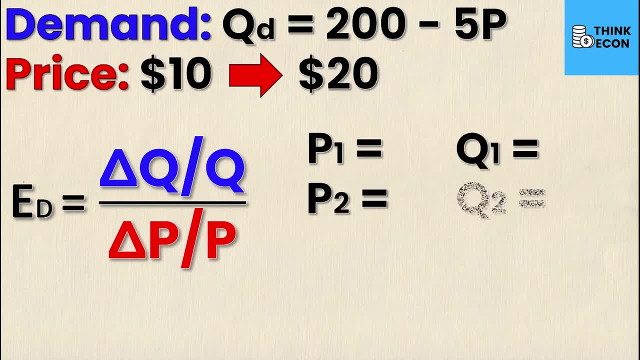 we're looking for a P1, P2, Q1, and a Q2.. That's just the old price, the new price, the old quantity and the new quantity. These are the key values that we need to find in order to calculate the 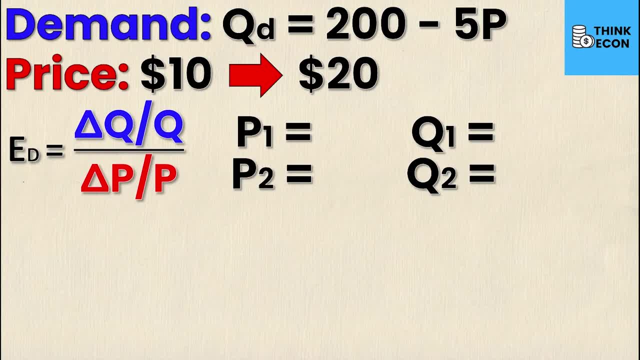 elasticity of demand. Well, luckily for us, the new P and the old P are already given and they're simply $10 and $20, and we know what they are because they're given to us. in the question, However, we need to calculate for the old quantity and the new quantity, and to do that we're 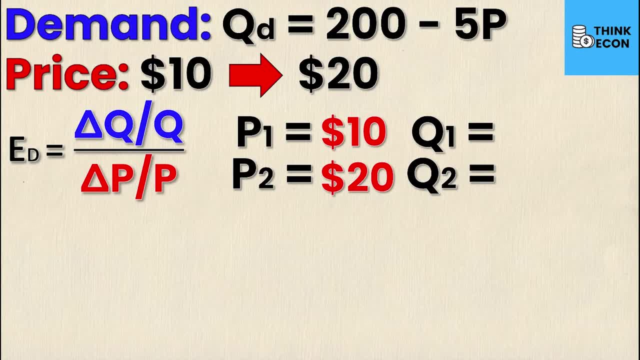 simply going to sub in the old and new prices, so P1 and P2, into the demand equation, one at a time, and that's going to yield us Q1 and Q2 respectively. So let's start with Q1.. We're going to sub it into. 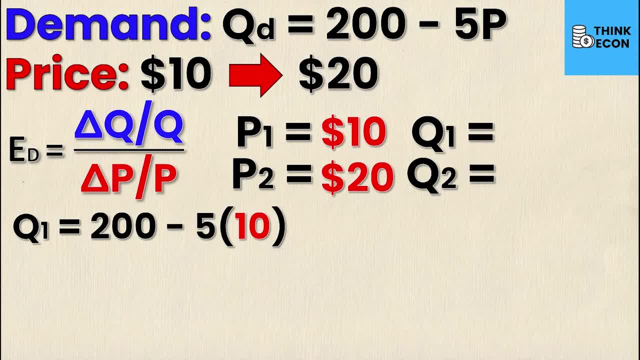 the demand equation that's going to give us: Q1 is equal to 200 minus 5 times 10.. Again, 10 is equal to 10 minus 5 times 10.. So that's going to yield us Q1 and Q2 respectively. So let's start. 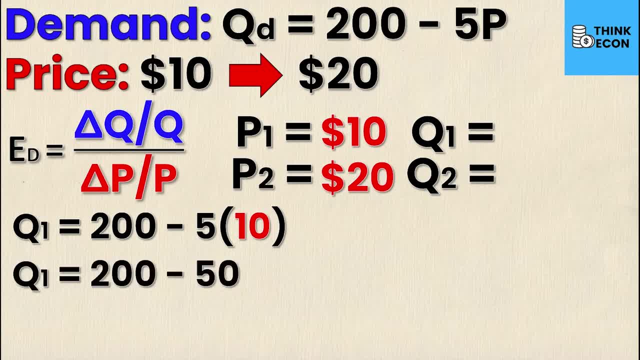 with Q1 and Q2 respectively. So let's start with Q1 and Q2 respectively. So that's going to yield us Q1 and Q2 respectively. So that's going to just P1.. Simplifying this further, we get: Q1 is equal to 200 minus 50, and then finally we can. 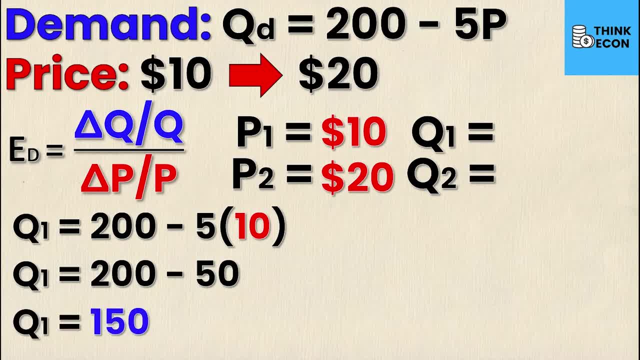 derive that Q1 must be equal to 150.. We'll do the same thing for Q2.. Q2 is equal to 200 minus 5 times 20.. 20 is just P2.. Simplifying further, we get: Q2 is equal to 200 minus 100. and then finally we can. 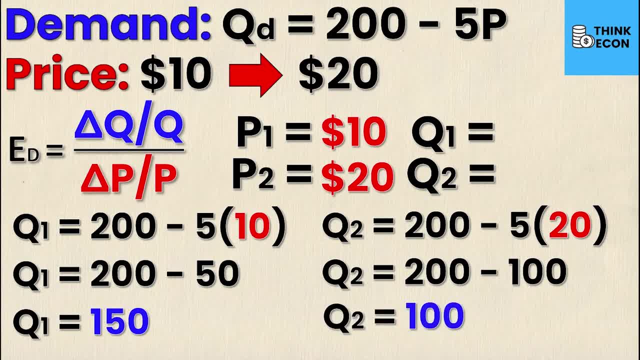 derive that Q2 must be equal to 100.. So now I have my P1, my P2, my Q1, and my P2.. So I'm going to P1 and my Q2.. Now that we have these four necessary values, we can finally solve for. 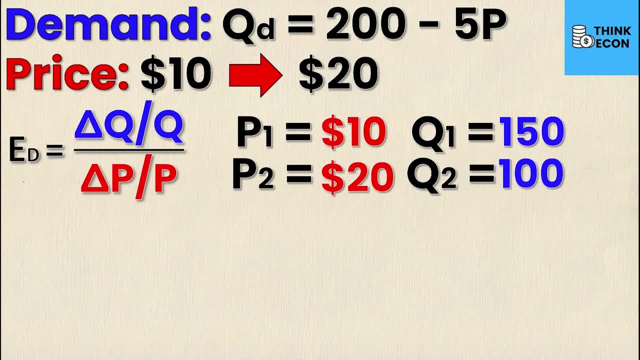 elasticity of demand. Now you might be looking at the elasticity formula saying that looks like percentage change, and it is. Now, if you want a detailed video on how to calculate all four types of elasticity, we have a video for each type on our channel, so feel free to check those out. We'll. 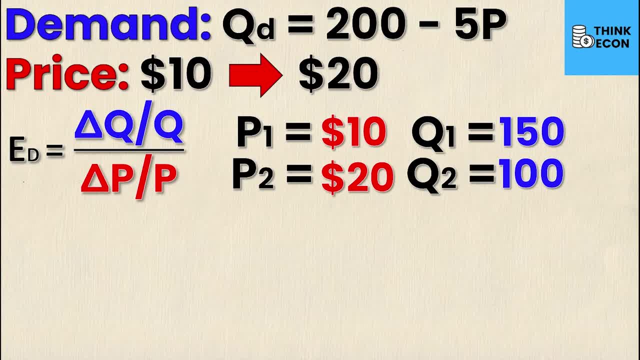 link them in the description To calculate percentage change. I'll explain it like I have in other videos. It's new minus old over old. That's the same as the change in Q divided by Q or the change in P divided by P. Let me illustrate what that looks. 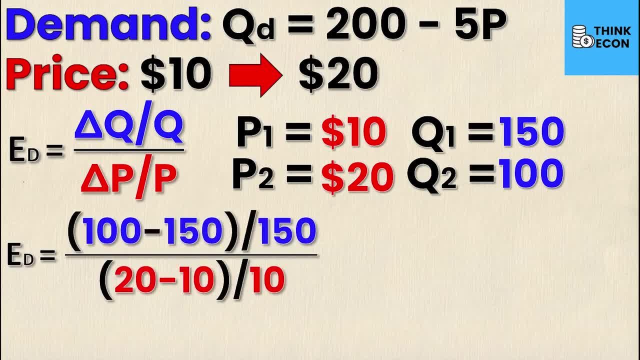 like with the numbers we have in front of us. So elasticity of demand is equal to the new quantity, which is 100, minus the old Q, which is 150, divided by the old Q, which is 150.. And I do the same thing for price: New price minus old price over old price. So 20 is the new price minus 10 divided. 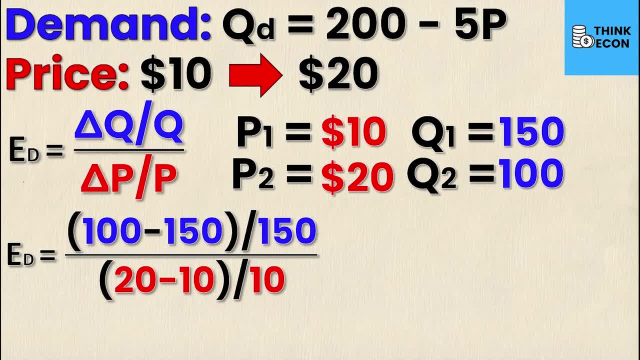 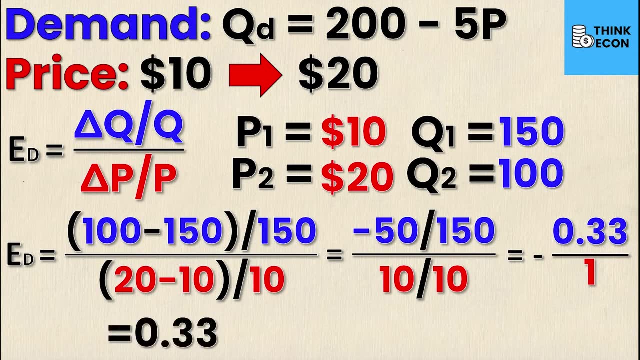 by 10.. That's the easiest way for you to remember percentages. So if I take the absolute value, as I want to calculate, the magnitude of elasticity is 0.33.. And you might be wondering to yourself: well, isn't the elasticity negative? And it is, but 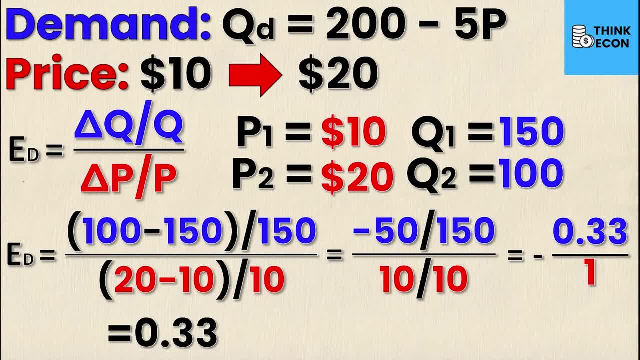 when you want to calculate if something is elastic or inelastic, you have to consider the absolute value, Because we know that the price elasticity of demand for a normal good will always be negative. So if I take the absolute value as I want to calculate the magnitude of elasticity, 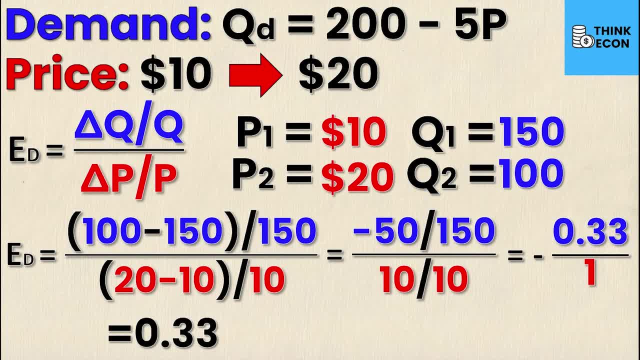 it has to be, because the relationship between P and QD is always negative. That follows the law of demand, where if you increase the price, then quantity demanded will go down. And that's exactly what you see here: Price goes up from 10 to 20 dollars and quantity demanded goes down from. 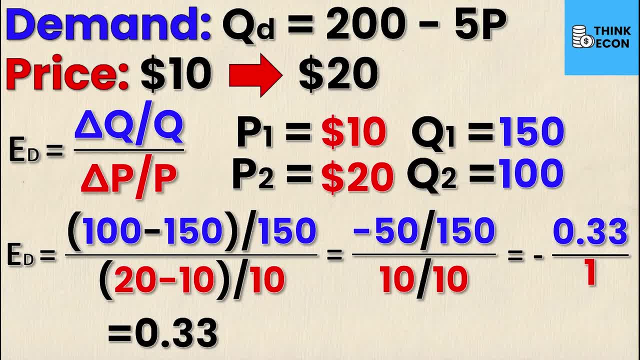 150 to 100.. So because those act in opposite directions, elasticity of demand for a normal good will always be negative. Anyways, assuming that you have that knowledge, we take the absolute value, which is 0.33.. That is 0.33.. So if I take the absolute value, as I want to calculate the,